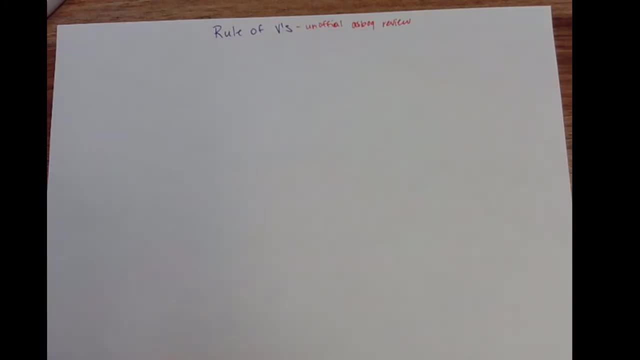 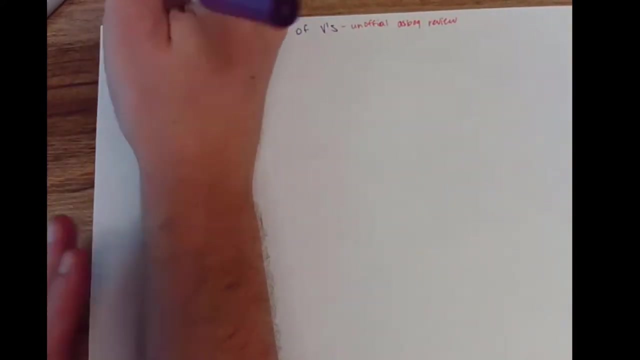 this exam and so going over some of the important concepts they might see in structure. So you might have heard the rule of these, but it doesn't always stick with people so well. So there are a couple aspects to the rule of these that you should memorize going into your exam- and I'm not a huge fan of memorization. 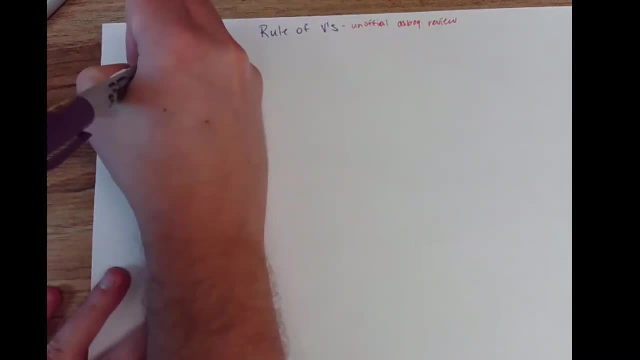 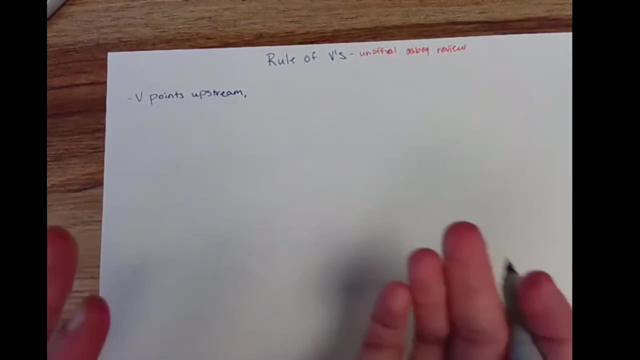 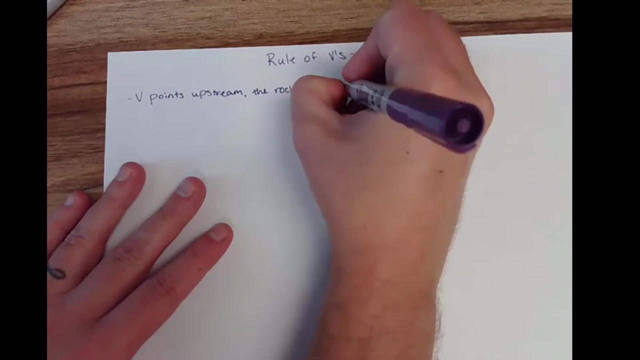 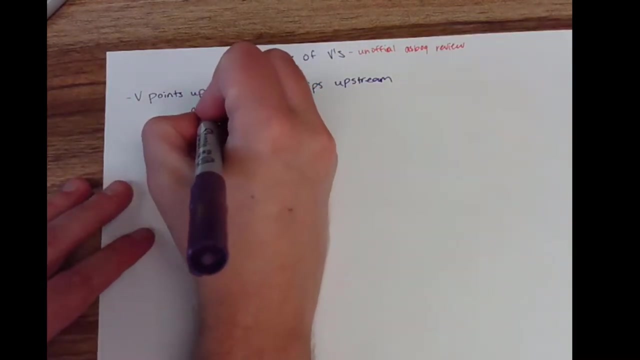 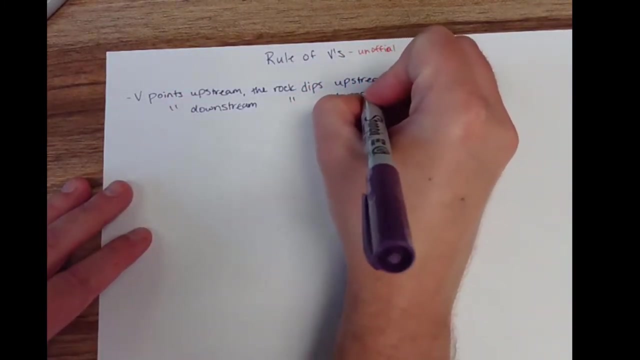 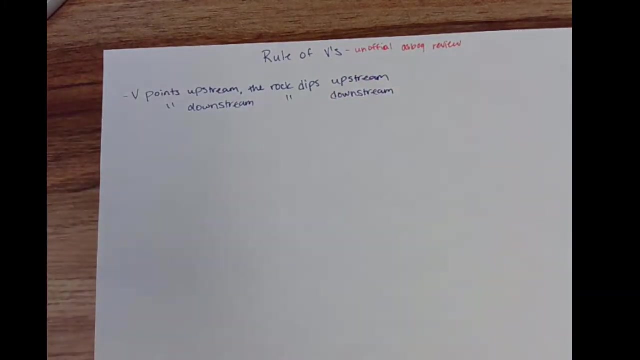 but here it is: If the V points upstream, then the rock dips upstream. The same is true for downstream. If the V points downstream, then the rock dips downstream. So that gives you an idea if the bed is dipping. Now, if the V gets really, really, 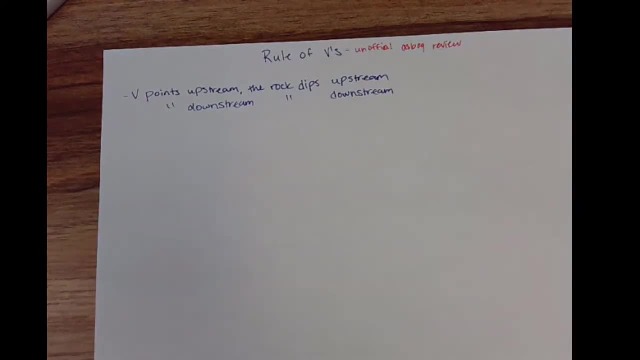 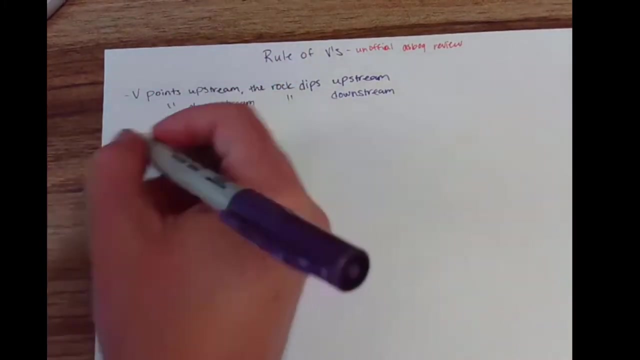 pointy, then that is going to end up being a bad grade, indicate a shallower dip. and if the V gets really flat, that's going to indicate a really steep dip. So we'll just write the extremes. So if the V gets so flat, meaning it opens up so much, 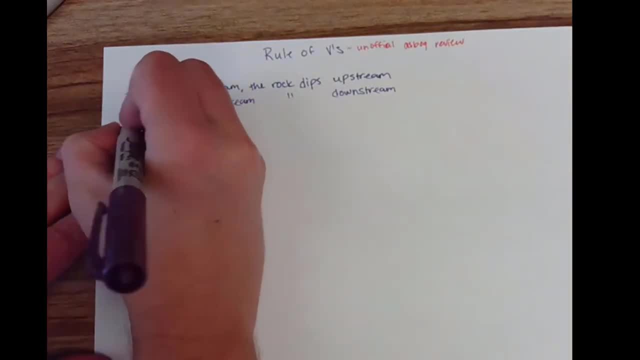 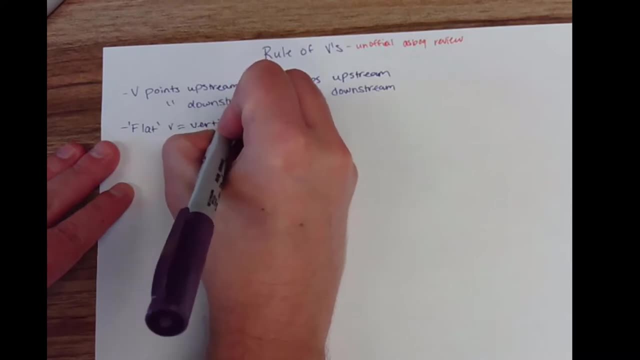 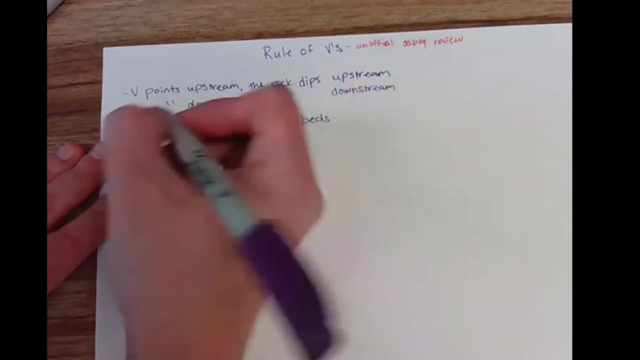 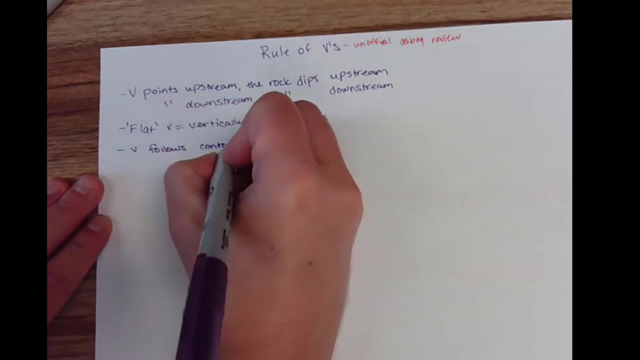 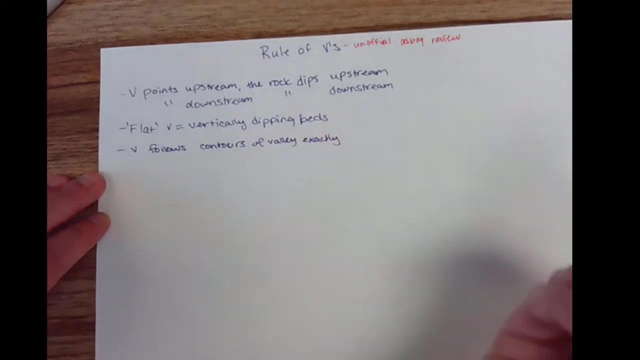 that it's just cutting across the valley, so we'll call that a flat. V is going to indicate that the beds are dipping vertically, And if the V follows the contours of the valley, exactly meaning the elevation contours, then your bed is going to dip zero degrees. 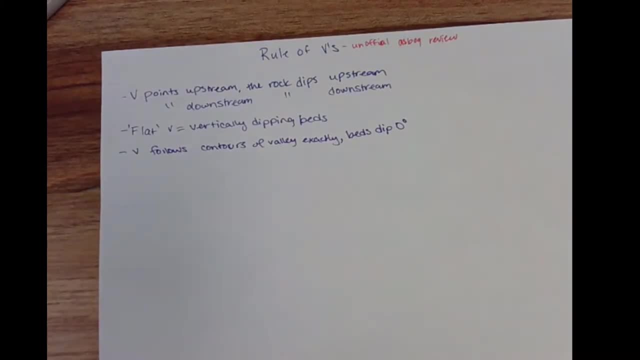 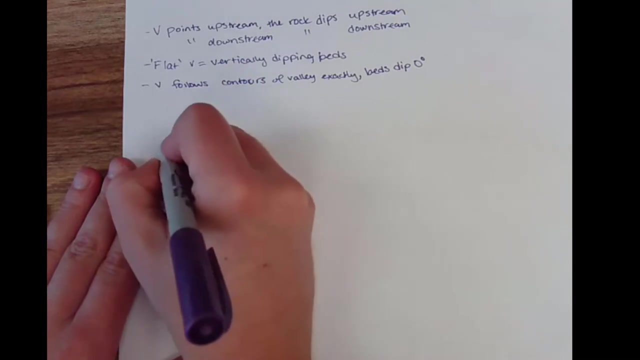 All right. So Those are the four things that going into this exam. I would bother to memorize about the rule of Vs. So let's just do a bit of sketching and figure out what this might look like. I tend to get an exam, have a little bit of anxiety. 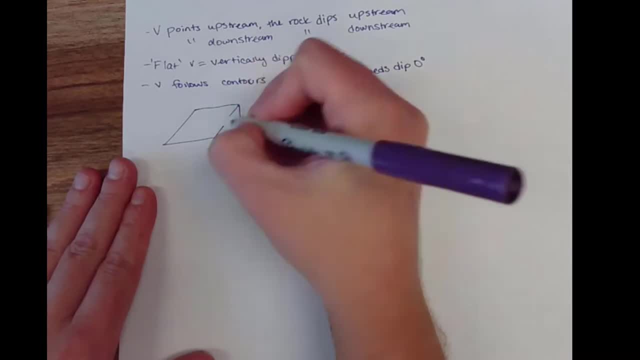 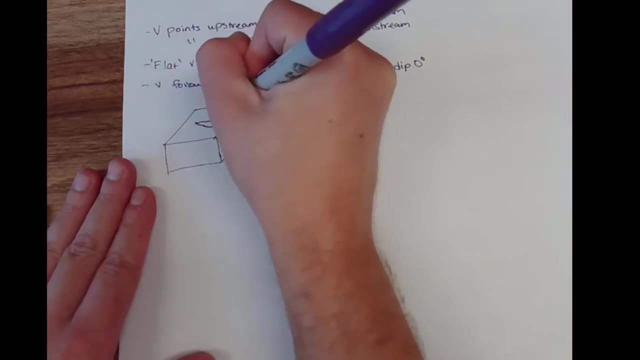 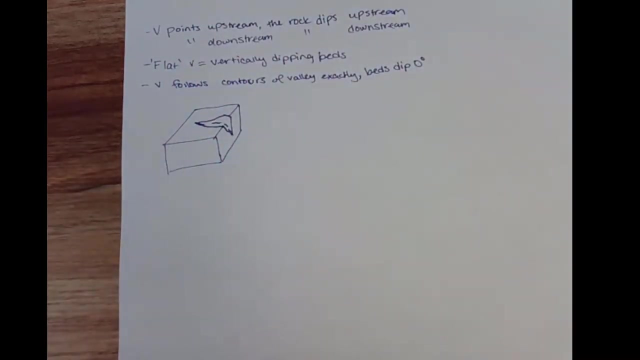 but drawing actually kind of calms me down. So sometimes if I don't want to memorize something, I'll just give myself a nice picture. I'll just say, okay, so here's my valley, I'm cutting into a block. 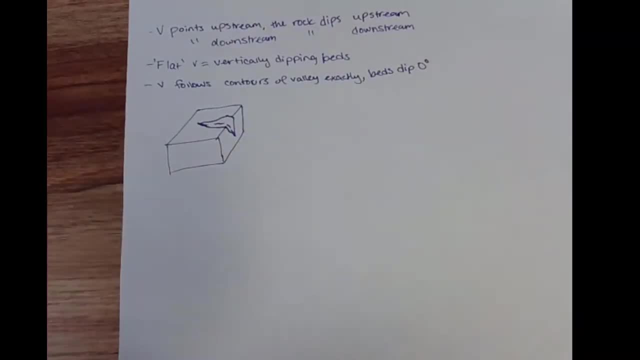 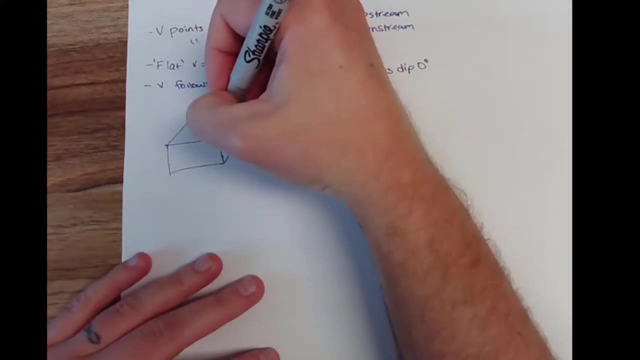 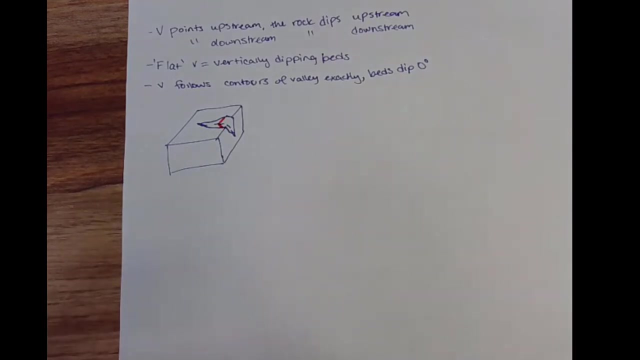 This is our front face, top face, side face, And let's say that we've got a unit doing this number. So you can imagine from top view that that is pointing upstream. So why does this rock then dip upstream? Well, as this V is coming up, it's going to be a little bit more. 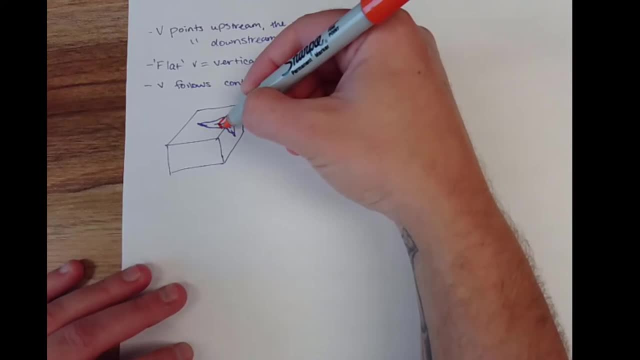 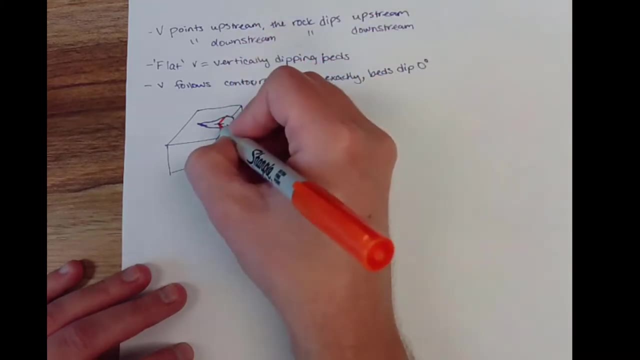 it's coming up to the side of the valley. It is coming up in elevation, So if this block is totally flat once that dipping unit hits the top of the valley, then we can imagine it coming straight across just like that wherever it meets the edge. 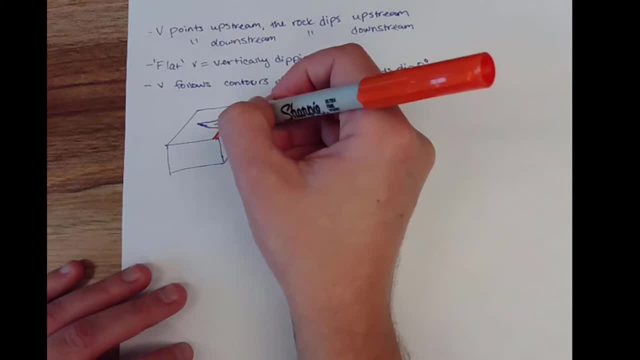 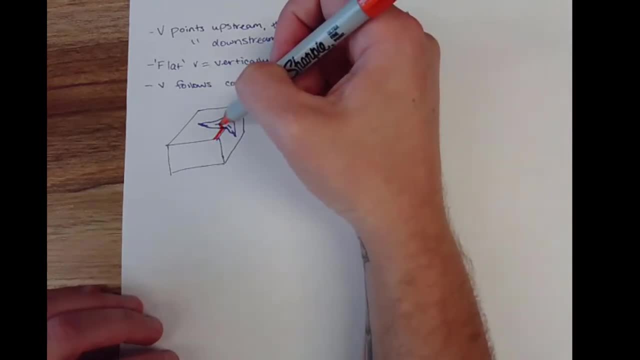 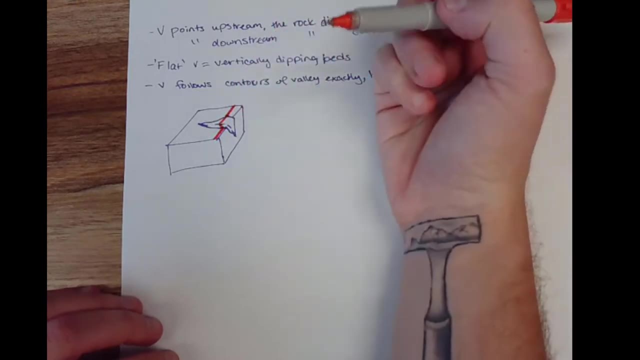 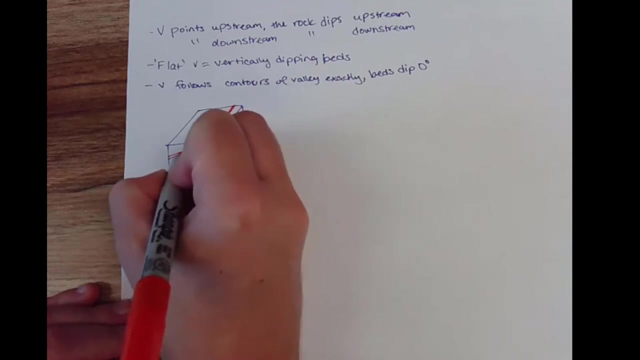 All right. All right, It's lower. You can kind of imagine walking down into the valley And, as you would be walking down into the valley and walking upstream, you're walking with that unit. So that rock unit is then dipping just like that. 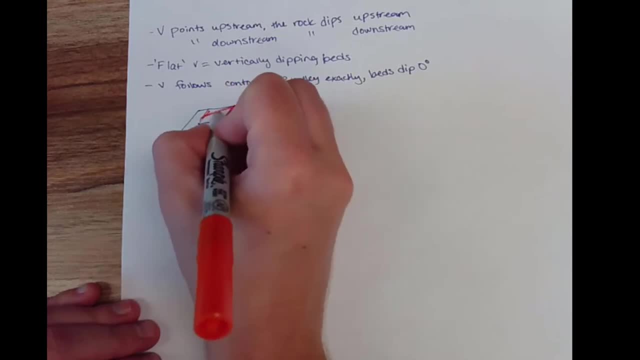 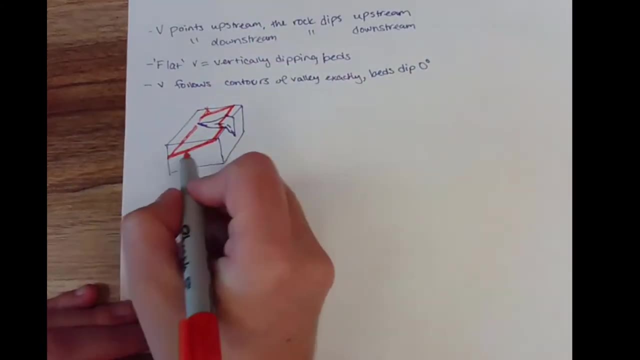 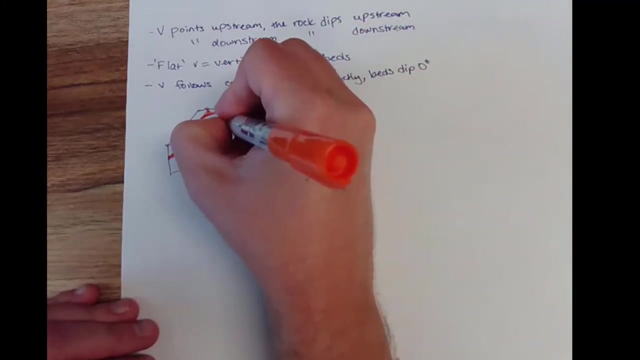 This is below the surface. Ignore that rock, Ignore that little piece right there. So that rock is dipping back and in The way that I drew this is I just drew this parallel, or tried to draw a parallel to that little side right there. 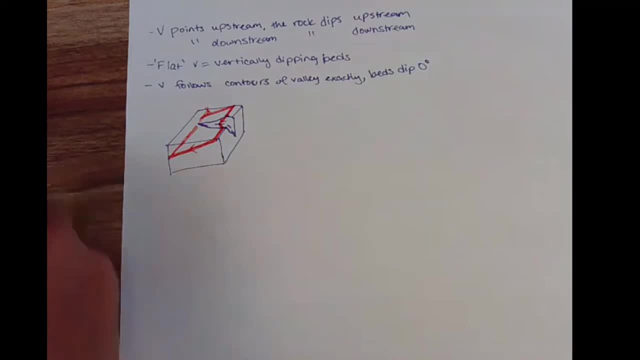 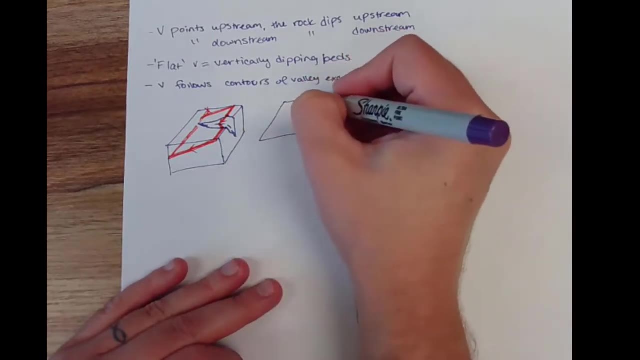 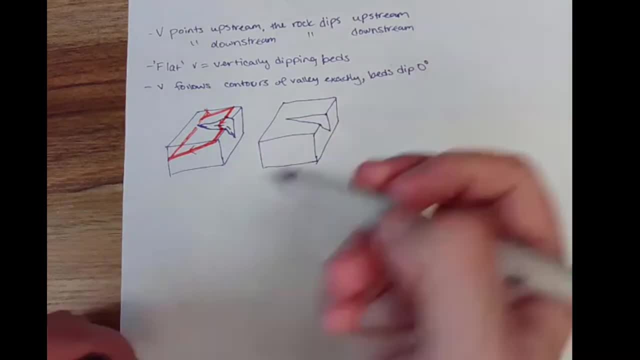 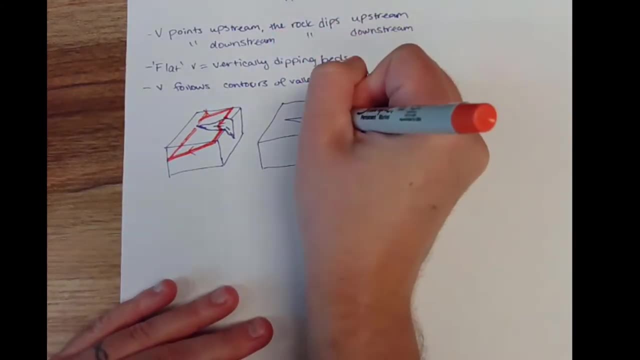 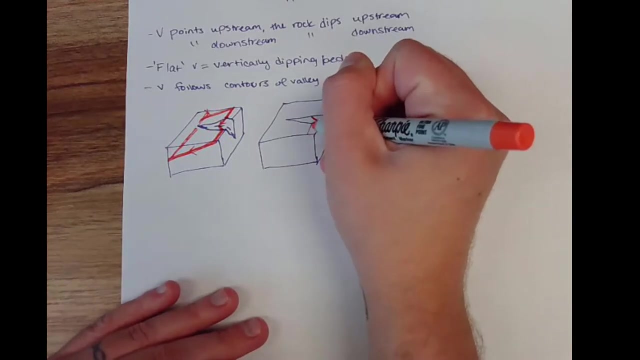 Here's our V: the surface expression of our valley, And we're going to imagine a rock unit that's dipping down. It's dipping in the same direction as the valley dipping downstream. We're going to do the same thing: Where it hits the surface, it would go straight across. 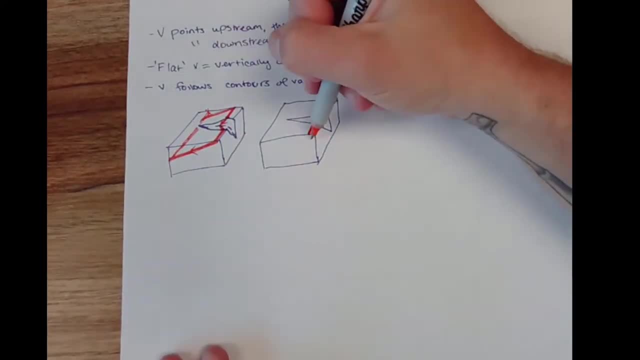 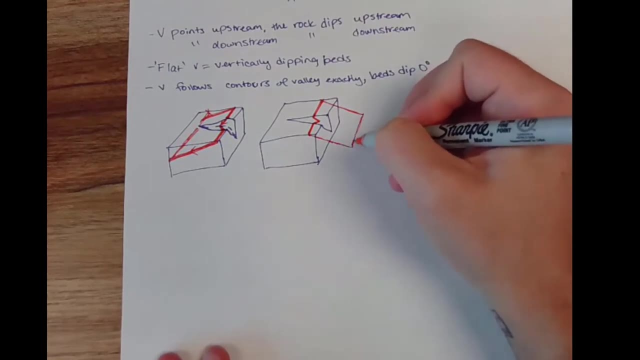 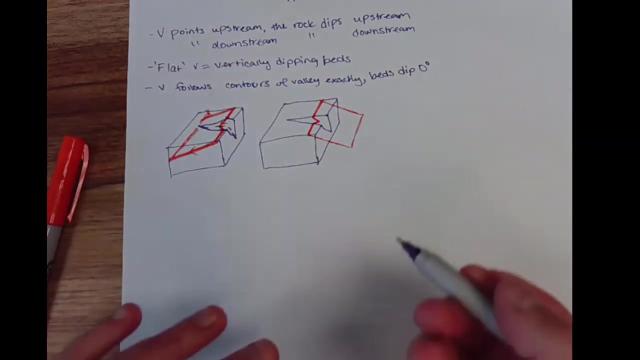 And then it has to follow that V, V at those angles. So here that rock unit actually cuts out and goes outside of our drawing so that we can draw that same plane. So here the V is pointing downstream and the rock as a plane is dipping downstream. Let's do the vertical. 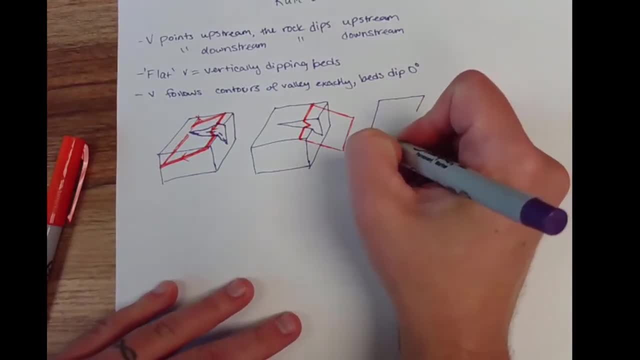 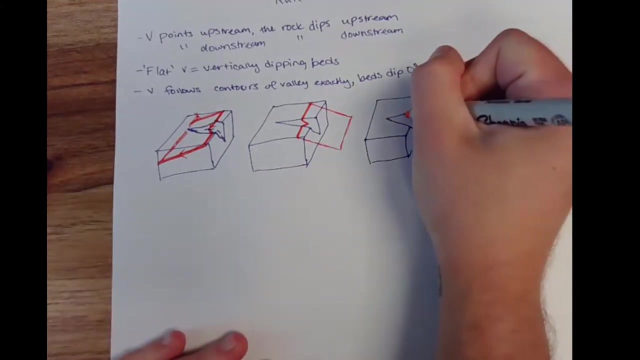 one. So now we're going to imagine that this rock does not care at all about the orientation of the valley, It's just going to cut straight across. So when it meets the side, it is also going to cut straight across. And when we try to draw, 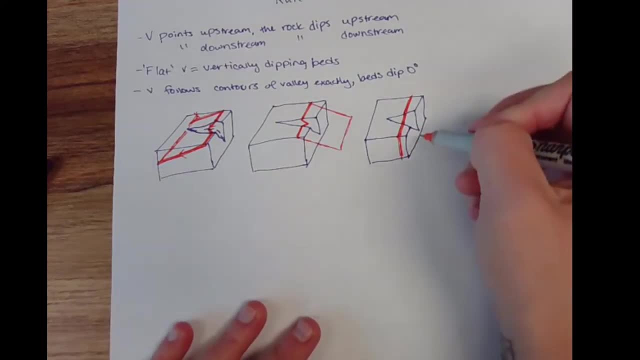 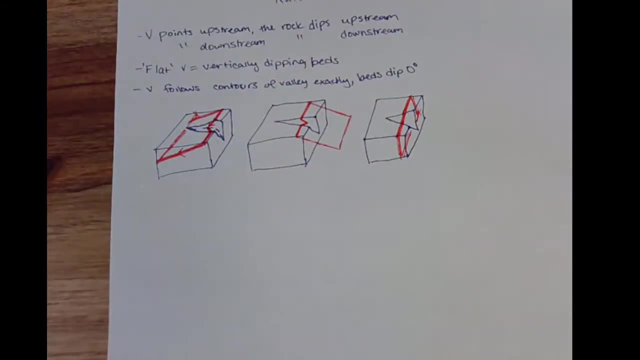 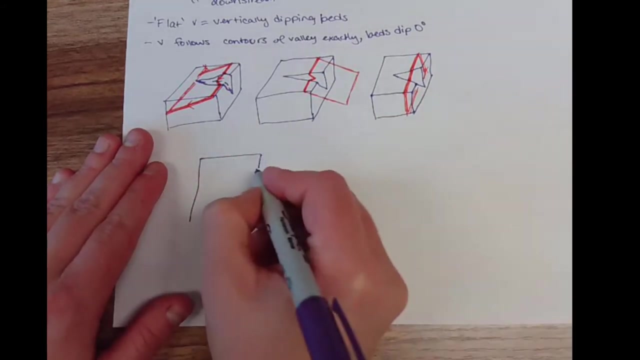 that in. we go kind of like this Imagine down here: So that plane is vertically cutting through the rock And let's see if we can't do a horizontal one. I'm going to have to draw my valley a little bit more open this time to get this, I think. Just so we. 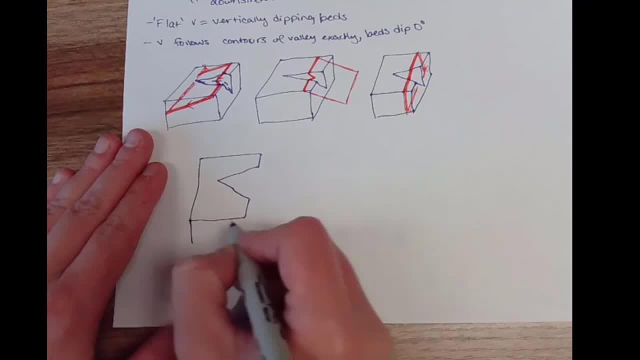 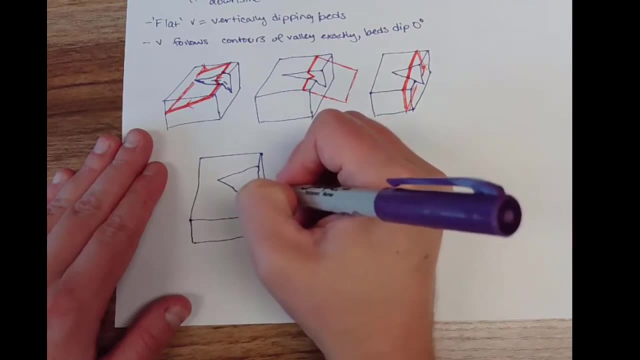 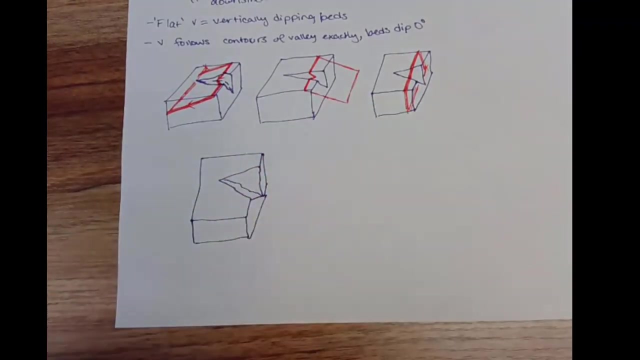 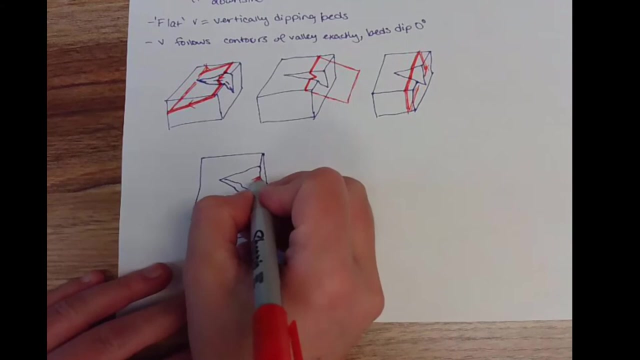 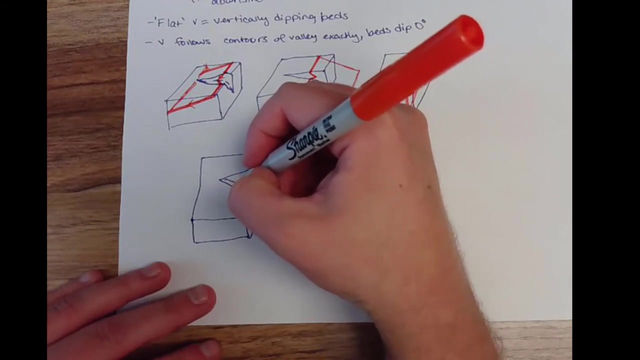 can see it better. My drawings are not perfect, but that's okay. Okay, Let's let this valley kind of follow, or the sorry the rock unit kind of follow the contours of the valley. So I'm just lining it up, trying to make it appear. 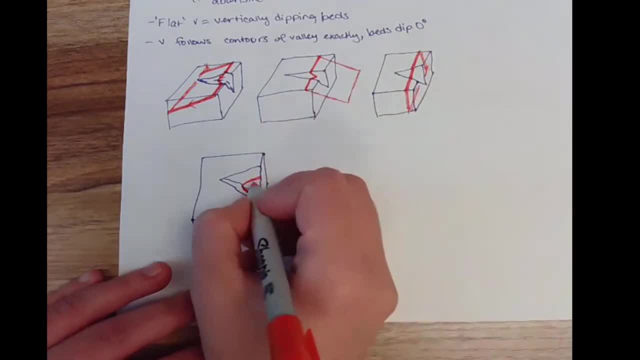 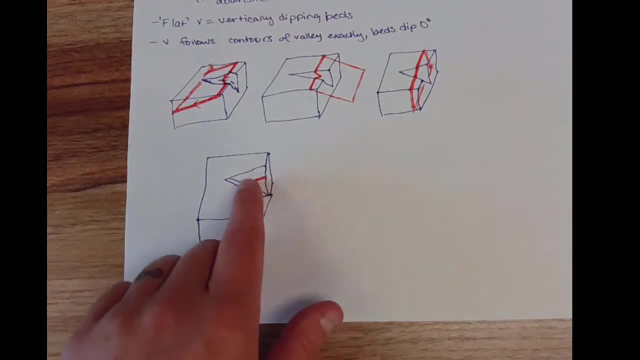 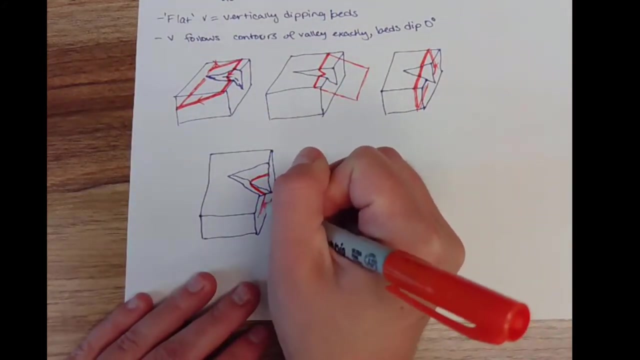 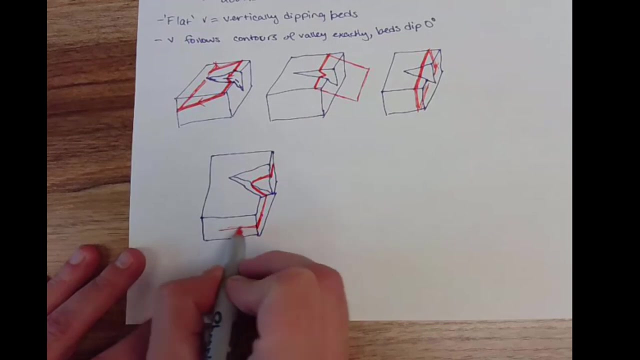 parallel to the sides as best I can. Got a little close on that side, but that's fine, Okay. So here the rock outcrop is following the contours almost exactly. So when I try to keep these going, they're going to actually hit the front side, not the top side this time, And I just keep drawing them where I can. 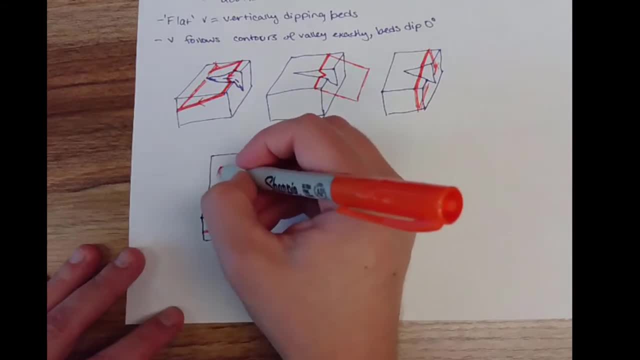 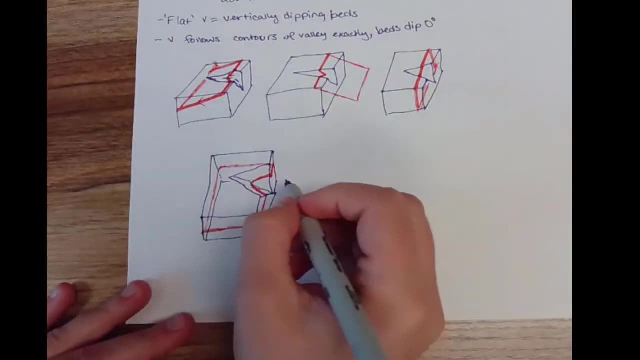 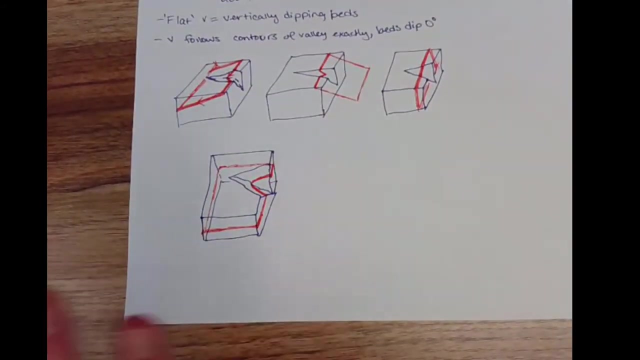 I'm going to go back through that side, Okay, Okay. So I'm going to go back through that surface And that's a horizontal plane slicing through that rock. So now let's mess with the expression of the V just a little bit. Let's take this valley and let's see if we can't steepen the bed that we have in it. 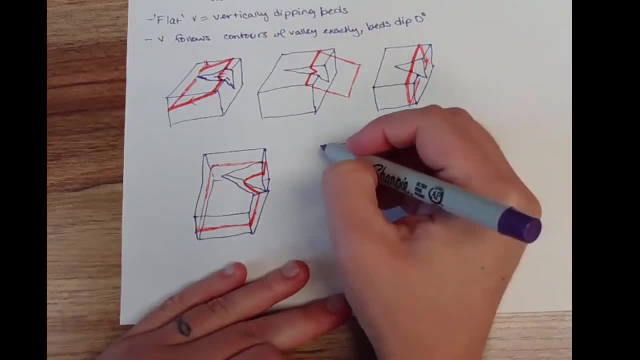 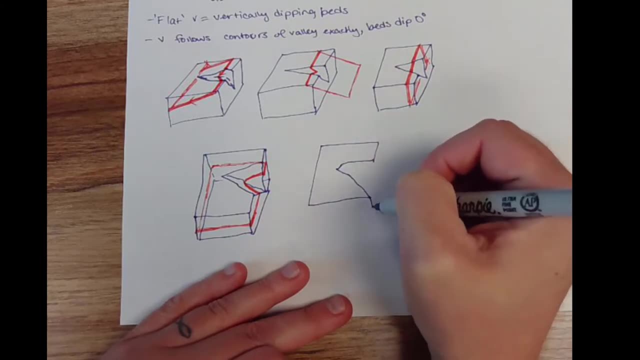 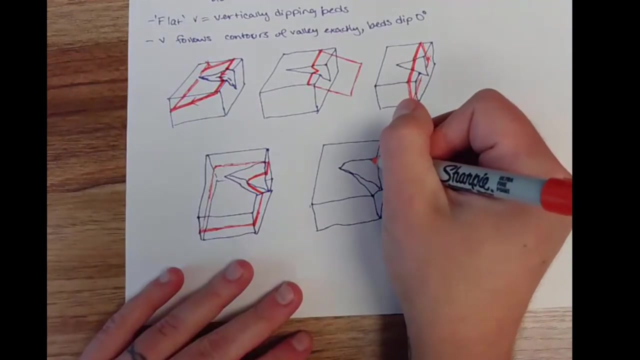 Okay, Okay, Wow, Oh man, what I did to myself there. I really opened that valley up, but I just want to be able to see this rock unit dip again. Okay, Let's make that V super narrow, almost like that. 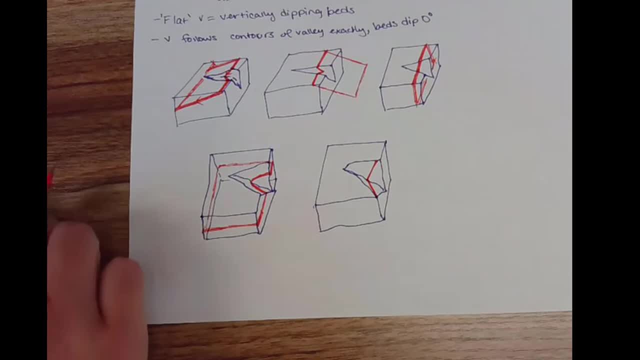 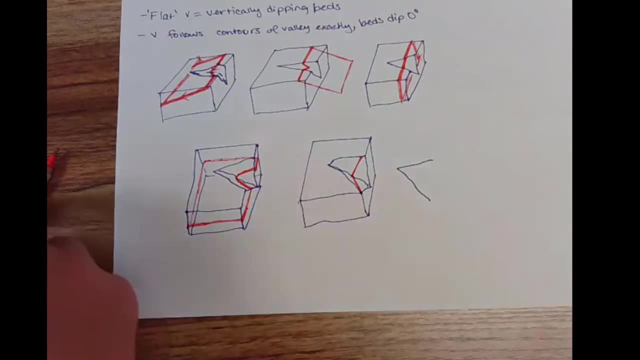 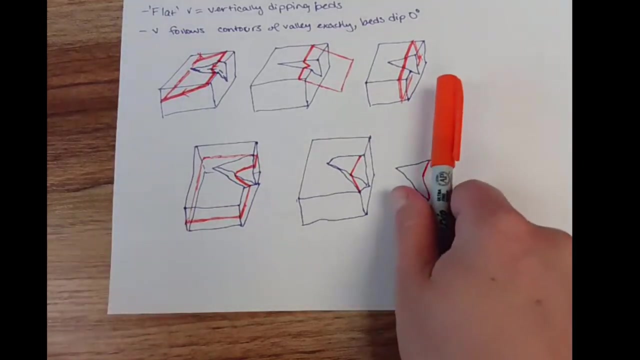 That you could. so, hopefully, what you can imagine is, if you're coming from the top, if you were looking at this, looking at this, you'd see this big, wide valley and you'd see a V kind of like that. so it's not quite a straight line, but it's got a really, really flattened. 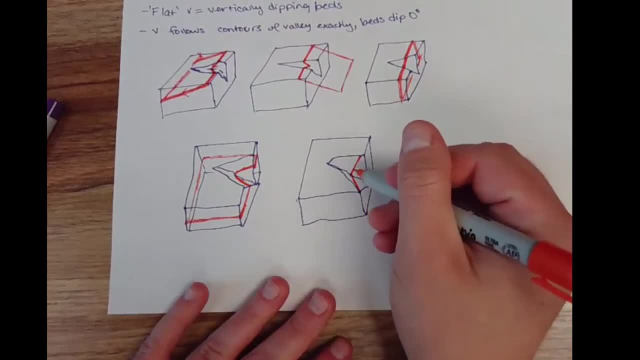 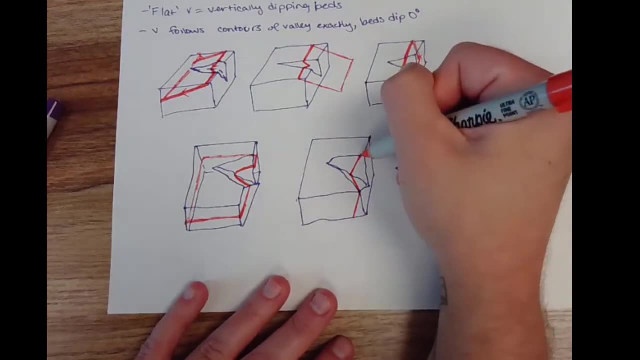 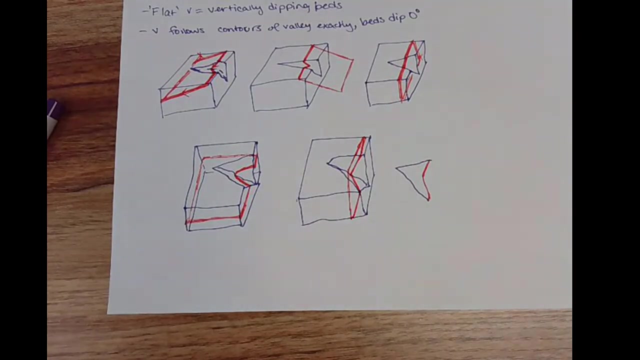 V shape. so now, as I try to keep my drawing parallel to these sidebar exposures- and it comes straight across because I'm at the top- this comes down, comes down behind that has a really steep plane slicing down through that rock. and we could do the same thing if we made the V. we go the other direction. 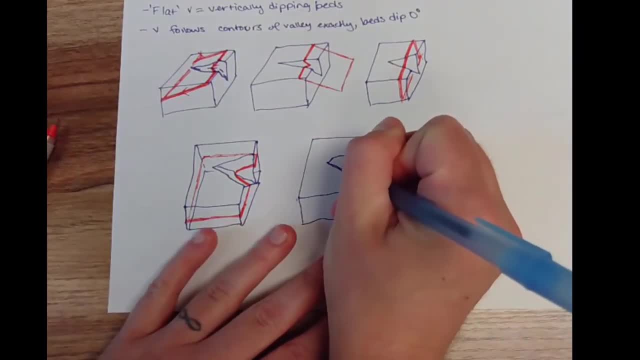 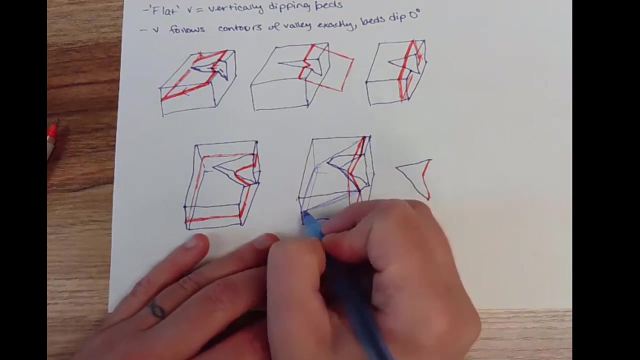 with this and make the view really pronounced, even more pronounced than the topography we'd still cut across here. but notice that if we try to stay parallel to this as we go back into our plane, we're gonna have to be really shallow with it, so I'll darken that in. 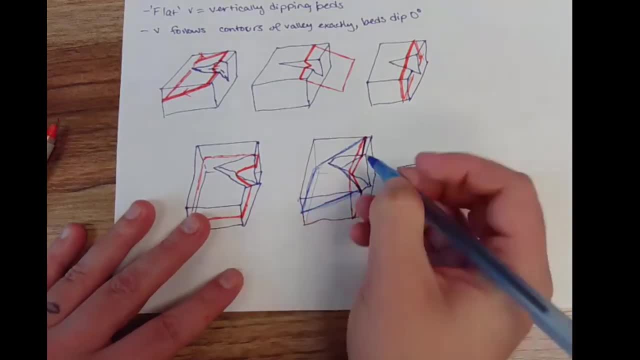 our plane we're gonna have to be really shallow with it, so I'll darken that in our plane we're gonna have to be really shallow with it, so I'll darken that in. so the more pronounced the pointy, or the V, the shallower the beds, because you can. 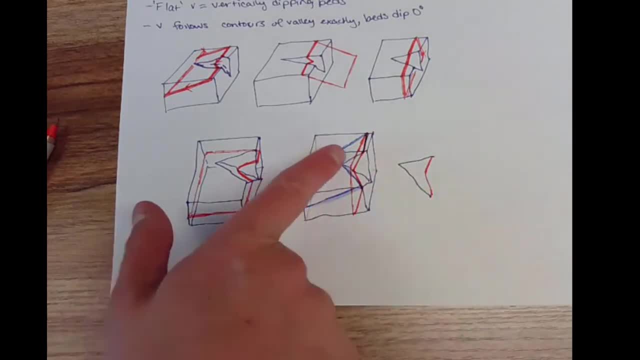 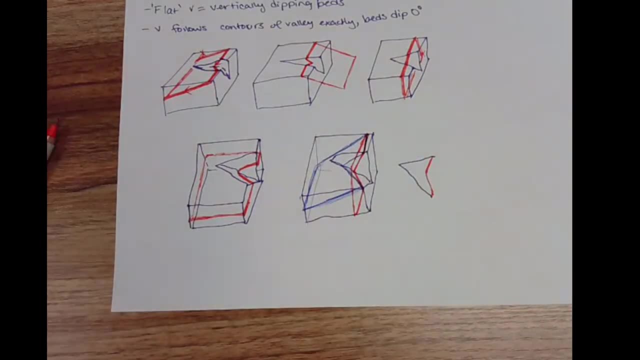 think about how that is basically trying to turn until it's following the contours exactly. so good luck with the rule of these.